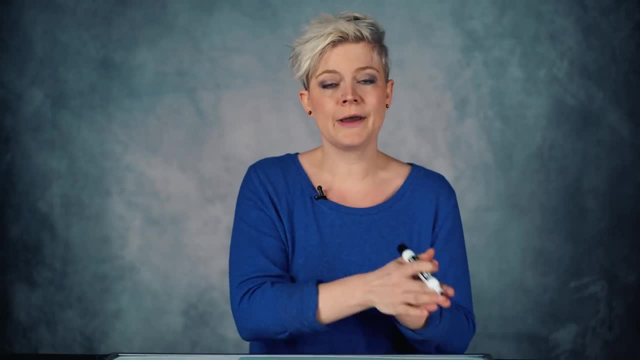 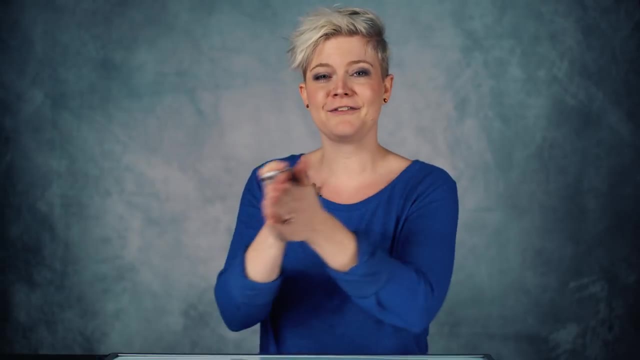 And if you were to clap this or count it, you would go one, two, three, four. Now the word half note is a two syllable word, so I find it really easy to go half note, half note, So you hold each. 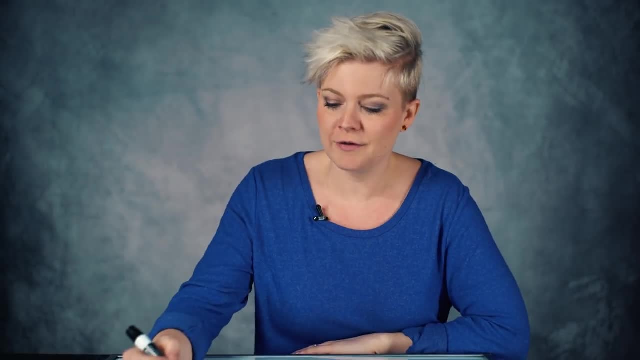 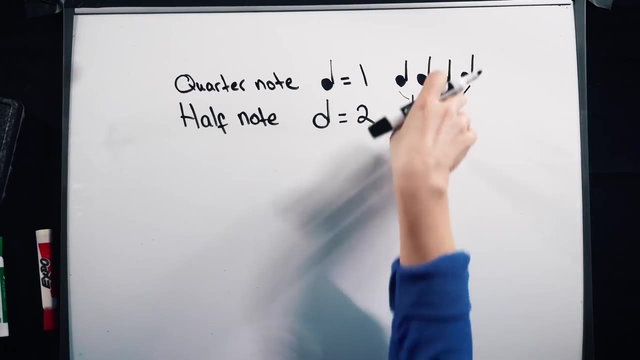 of those half notes for two counts. Now here's a cool little piece of information. Each half note could fit two quarter notes right, Because two quarters put together makes a half. So you can see how this kind of funnels into each other. The next note I'm going to show: 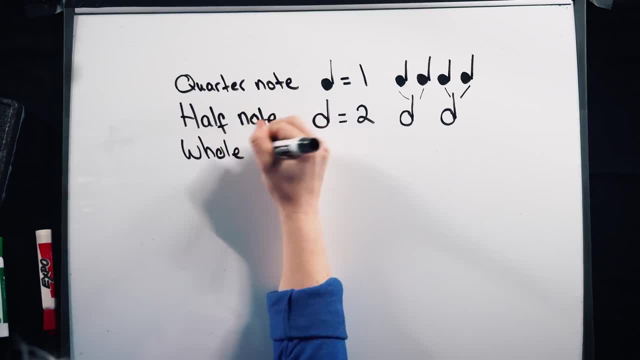 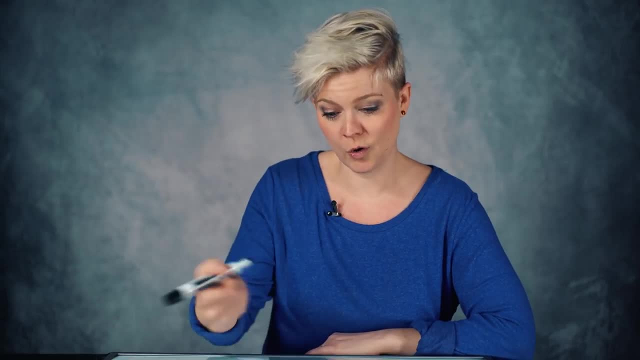 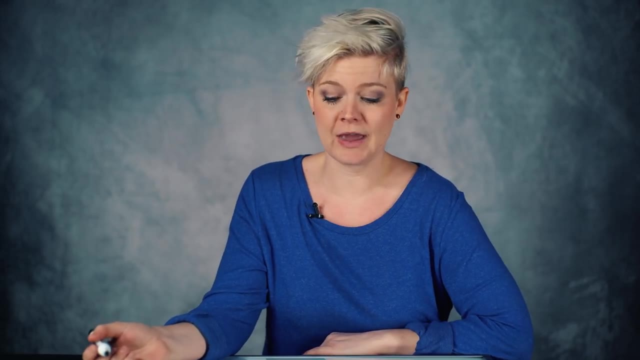 you is the whole note. So this one's pretty straightforward. It looks like a circle- You can maybe think of it as like a donut hole or a hole, And it equals four beats. So that's an entire measure of music. If you have a whole note here, you're going to count it like this: You're going. 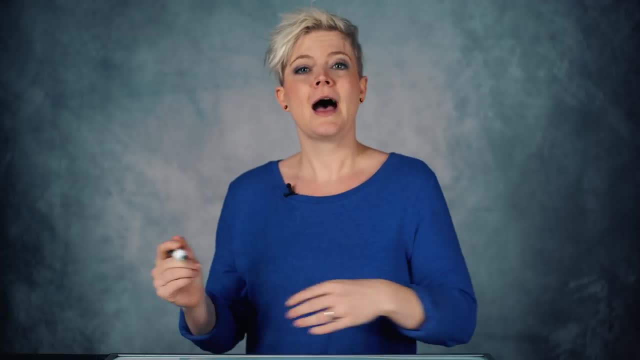 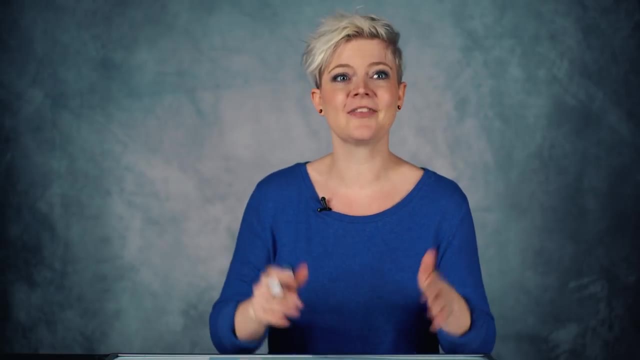 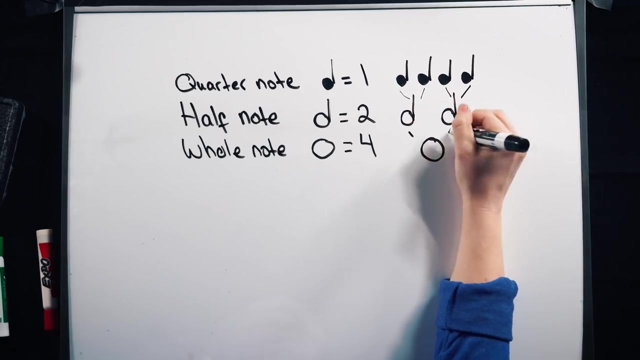 to go one, two, three, four. I like to say great big whole note because it's got four syllables and it helps me to remember the value. So you could count it like this: So great big whole note, One clap and four beats, And we could fit two half notes into one whole. 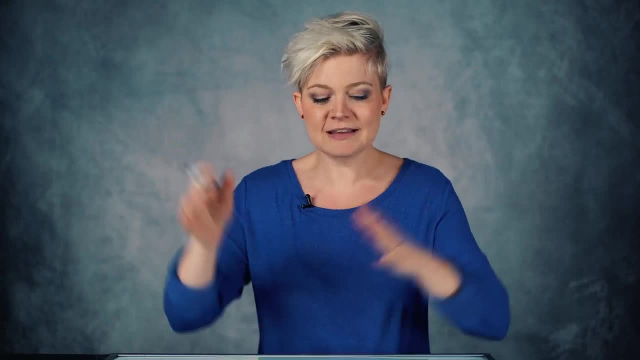 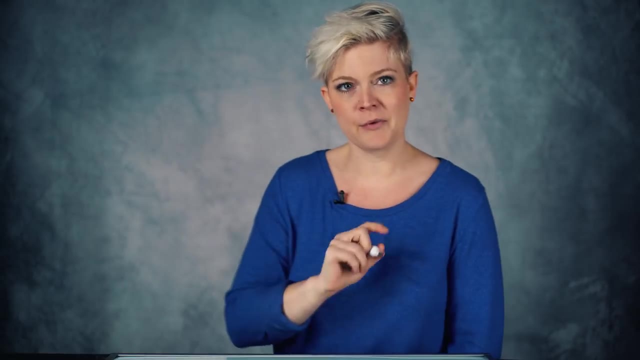 note, or four quarter notes into one whole note. So that's like the most basic, simple look at rhythm. We have more note values that we can add on to this, So let's take a look at one of my favorites. This guy is called the eighth note. Now it's really, really fun. 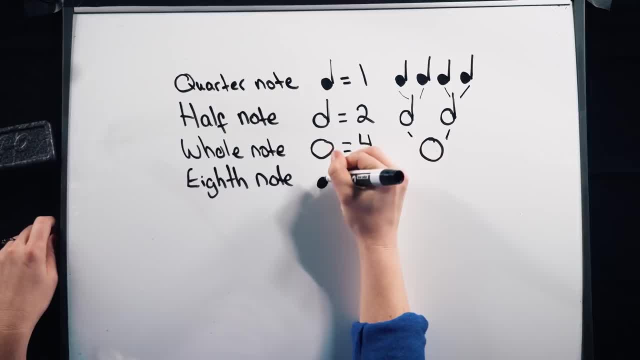 to draw. It's a really common one. It's called the eighth note And it's a really, really easy one. you know, when you're sort of doodling notes Colored in like a quarter, but it's got a little stem like that And this little guy equals one half of a beat. So that can. 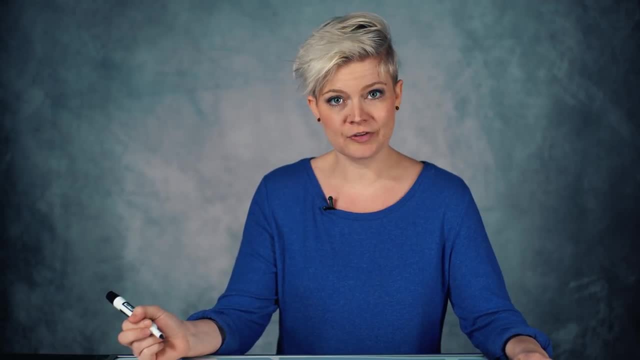 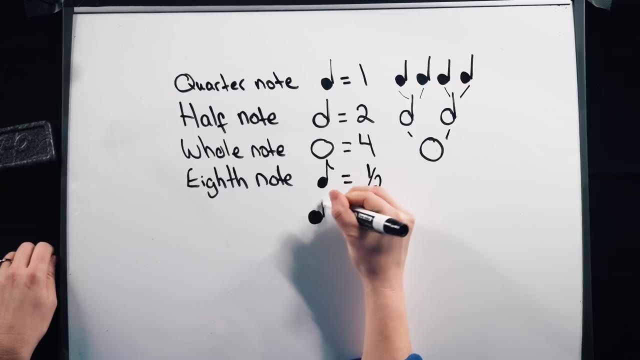 get complicated. So we often see eighth notes in groups of two. So when you put eighth notes beside each other, instead of having their little stems point down like this- I'm going to show you this right here- Instead of those downward pointing stems- we actually can't. 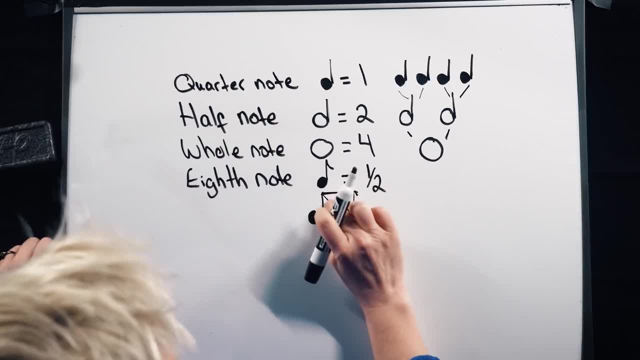 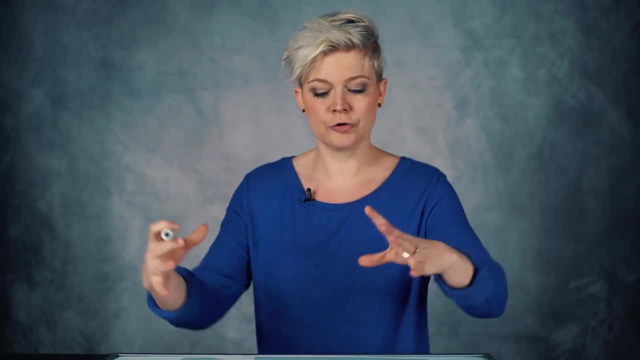 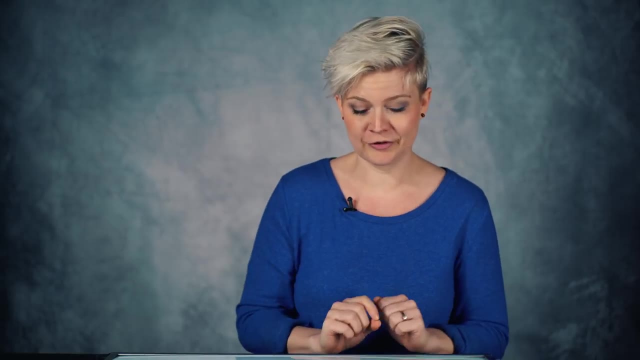 get mixed notes. We actually connect them like this: We're going to erase those stems, And that's what you get. So you get two notes that put side by side, equal one. So they're grouped together in groups, which makes it much easier to count and to read. So eighth: 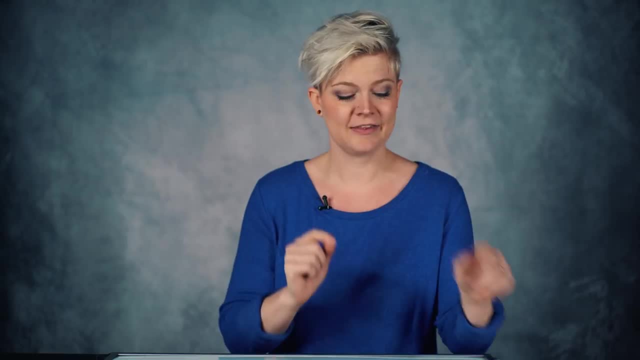 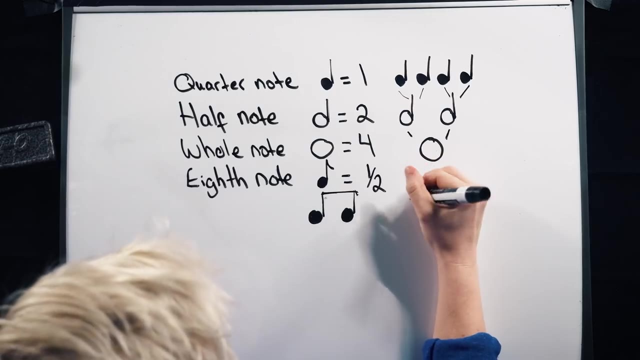 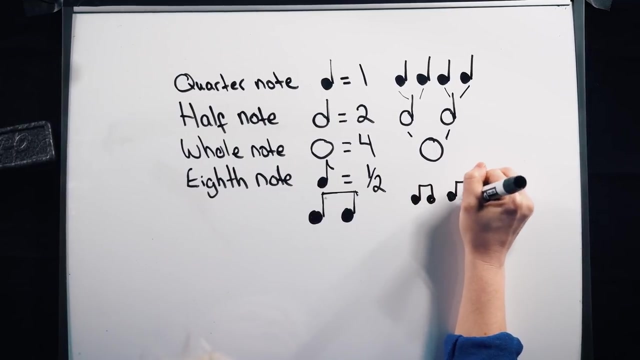 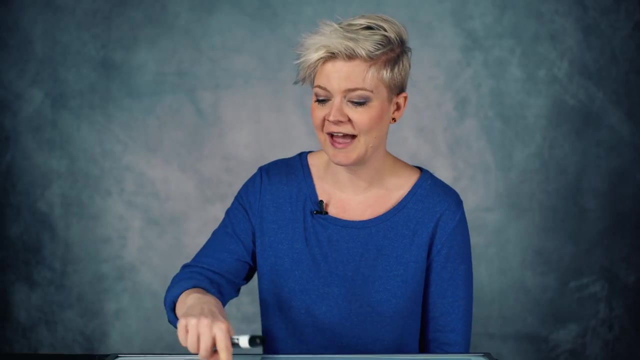 notes are often counted like this: One and Cause that breaks those ones into half, so you can count single eighth notes or eighth notes together. So I'm going to do a group of 1,, 2,, 3,, 4 beats Notice I have 8 notes. So we count it like this: 1 and 2 and 3 and 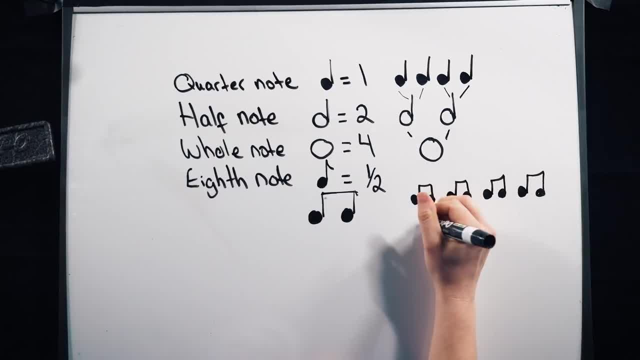 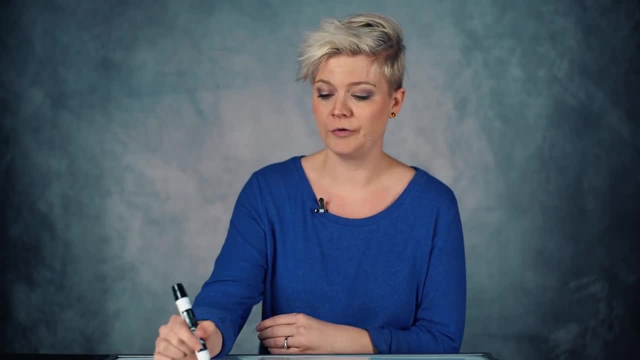 4, and So this is 1 beat, this is 2, this is 3 and this is 4.. So all of these guys together equal a whole note, or 4 beats, 4 quarters. So I hope you're tracking with me so far. 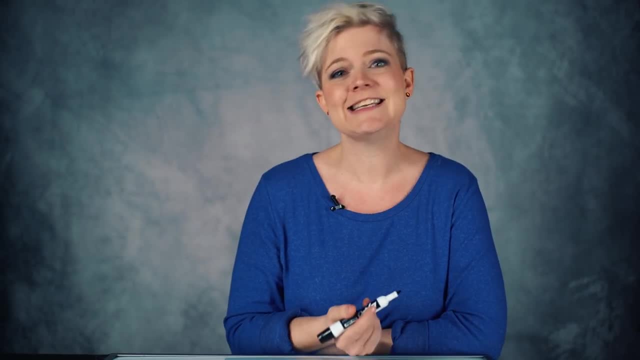 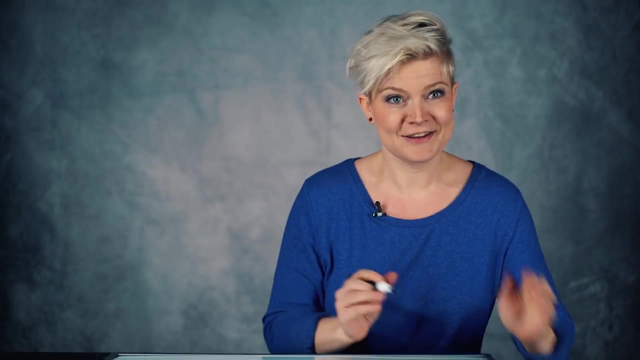 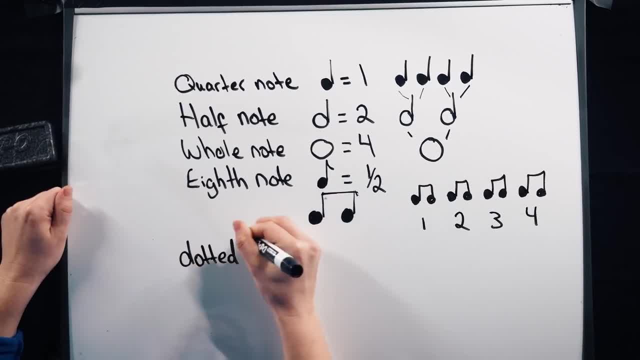 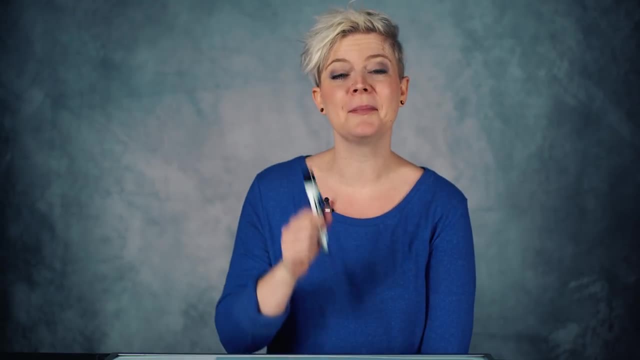 here we're going to use a dot, A dotted half note. So we're going to take a half note and we are going to put a dot beside it, So we've got a dotted half note. Now, any time you add a dot beside a note, it adds half the value. 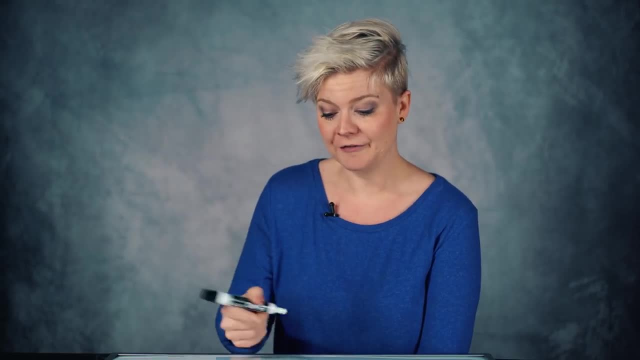 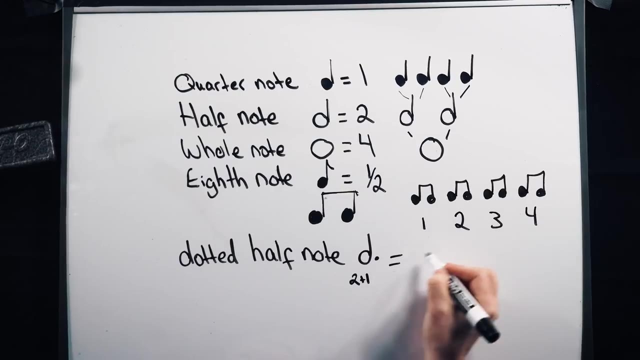 of the note. it's beside to the note, So a half note equals 2.. Half of 2 is 1.. So we're going to add that, giving us a note that equals 3.. A half note dot equals 3 beats. So you. 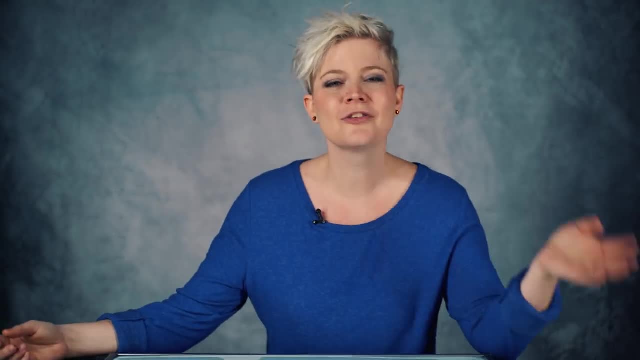 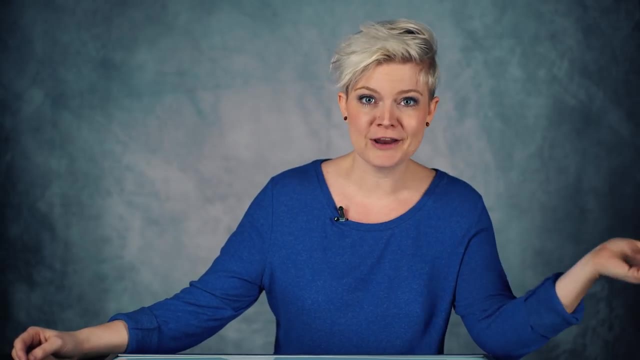 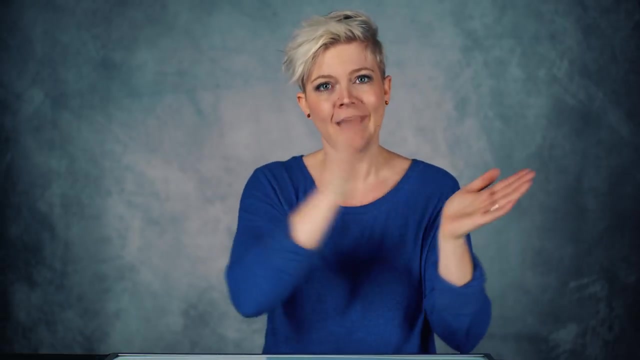 could count it Half note dot. See, I just called it a half note dot. there It's grown up name is a dotted half note. But if you say half note dot, you get those three syllables, which helps you to remember the value of the note. So that's how I count my dotted half notes now Half. 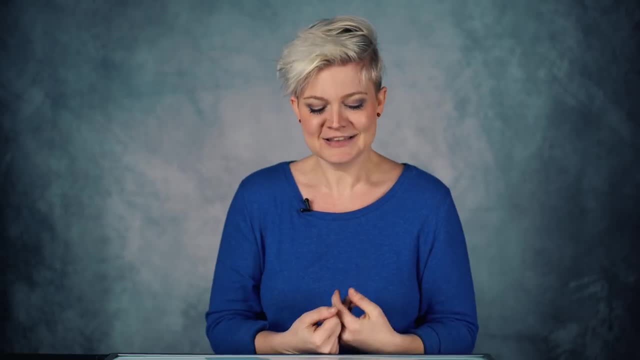 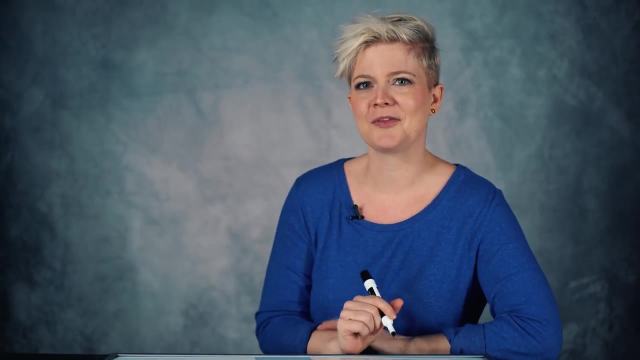 note dot, Or 1,, 2,, 3.. So a dotted half note is a lot of fun. Finally, this is the last one. It's maybe one of the more complicated ones, but when you break it down this way, 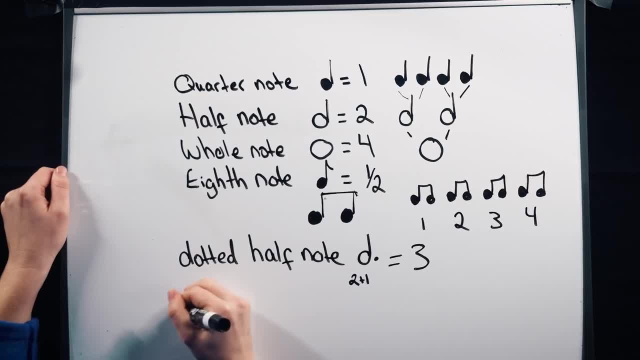 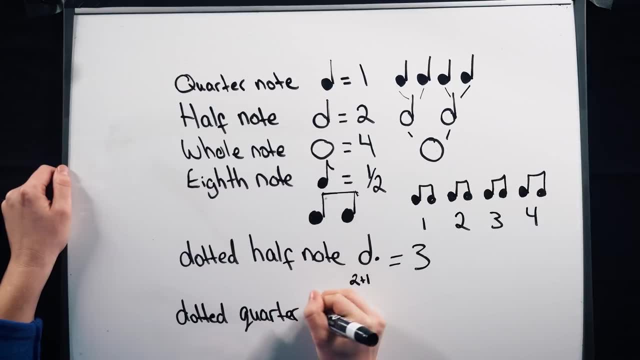 I find that it makes the most sense. So what it's called is a dotted quarter note, And it sounds simple. All we need is this lovely little quarter note guy here. I'm going to put a dot beside him, But we need to figure. 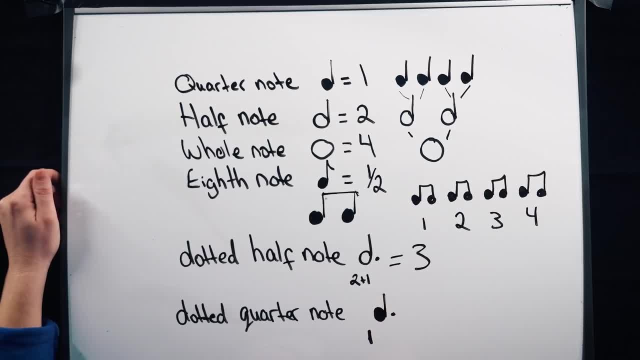 out the value. So a quarter note equals 1.. We're going to add half the value of that 1 to the note. So we're going to add half of 1, which is 1.5.. So now we have a note that. 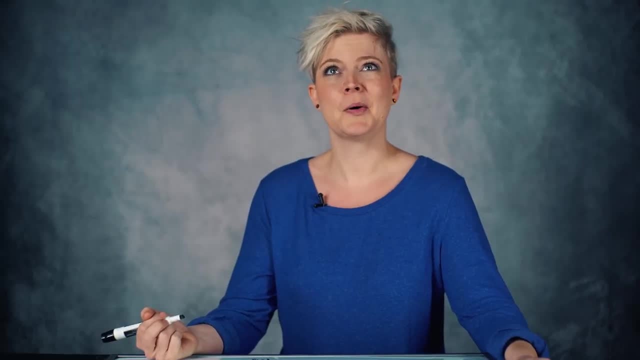 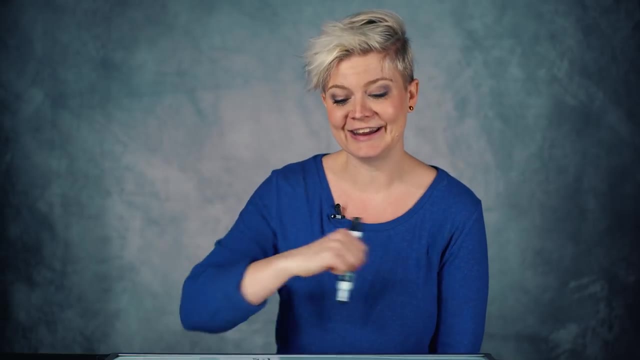 equals one and a half beats, And that's kind of something you can't leave alone. You have to complete it. So we're going to find something else that we've learned in here. that equals a half a beat. our friend, the eighth note. 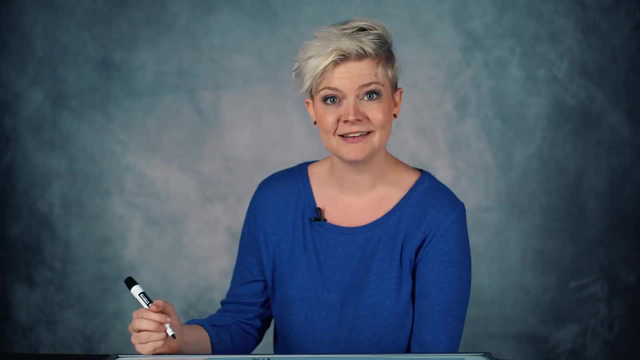 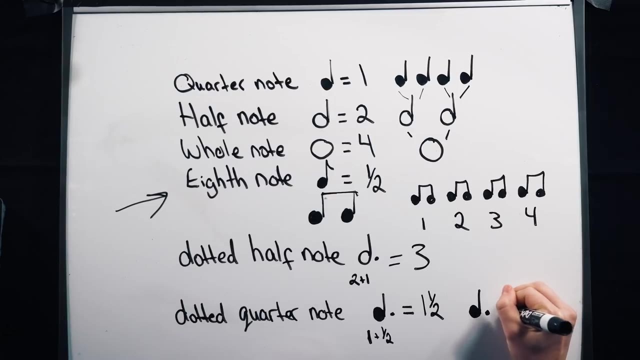 and we're gonna use that little lonesome eighth note to complete the value. So when you see a dotted quarter note, you'll almost always have an eighth note in the same measure. So we've got a full beat here for the quarter. 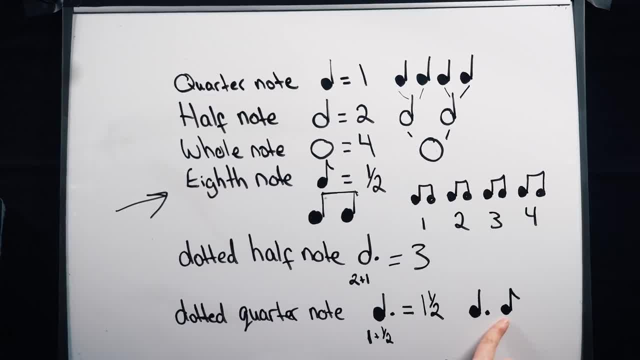 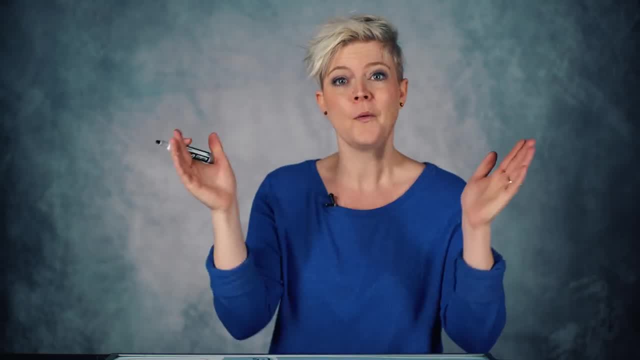 a half beat here, and then this little guy here is also a half a beat. So together this would equal two. So it sounds like this one and two and Another way you could count that, which again, it's silly. I use this in my kid classes. 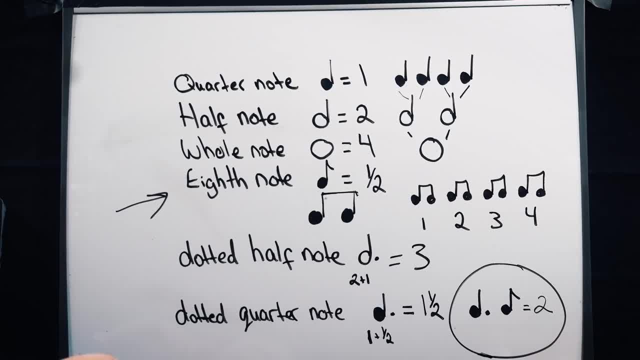 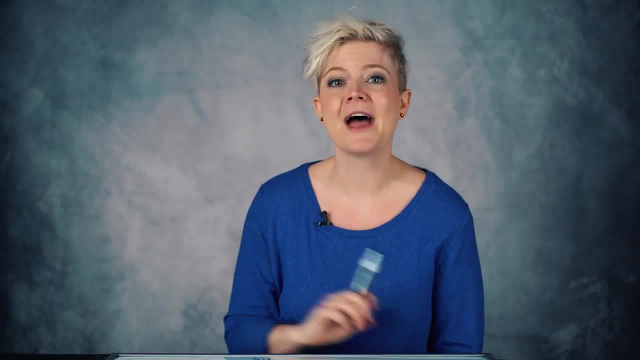 but I find it really helpful. I call the quarter note a ta, and then I call the dot a dot, and then I call that eighth a T. So I go ta dot T. So whatever way you wanna look at it, go for it. 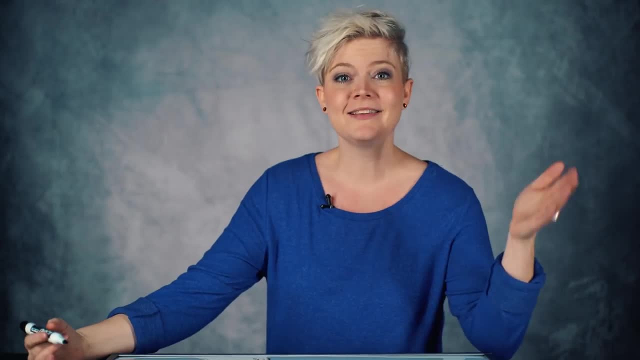 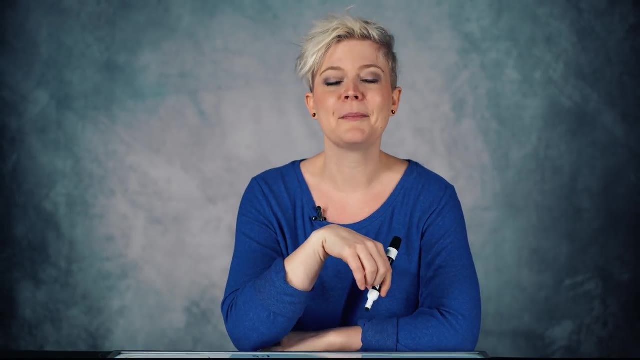 This is an overview on note values. what the notes equal. Write these down on a piece of paper and see how many of them that you can memorize. Make little combinations of the different note values and practice clapping them. It's really, really gonna help you. 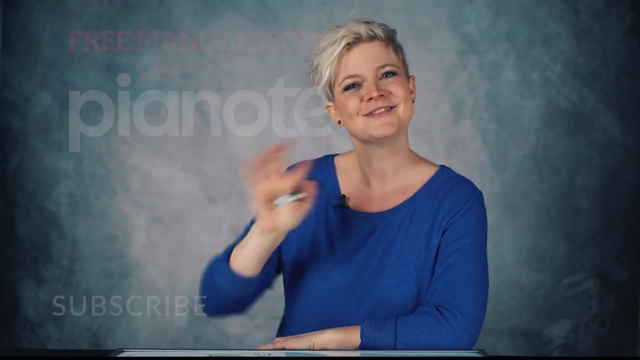 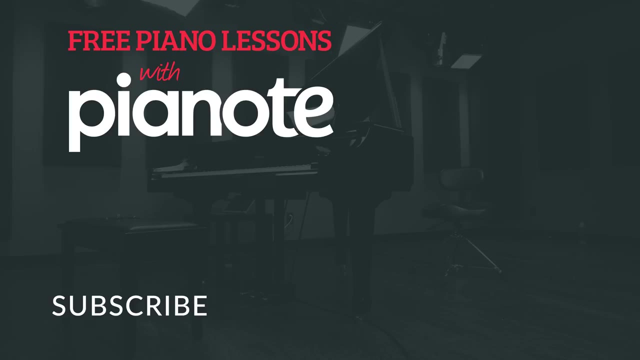 as you learn to sight, read and play. So enjoy this lesson and we'll see you around. Captions by GetTranscribedcom.